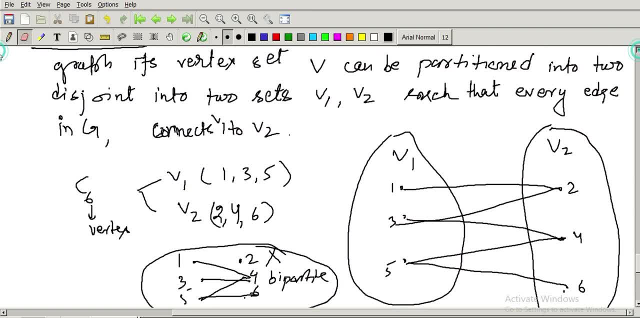 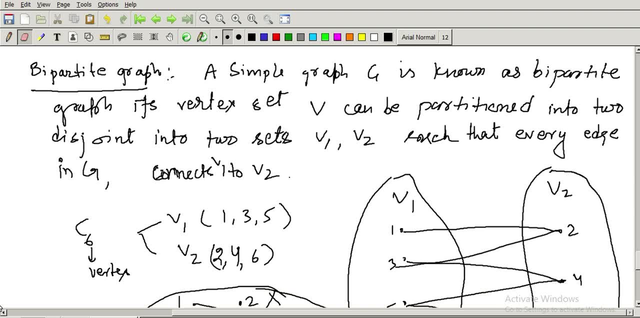 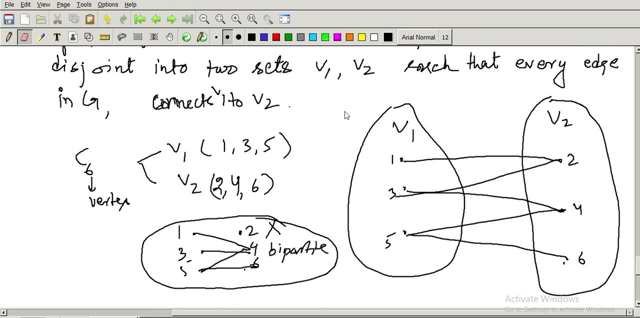 And in the last lecture we were discussing about the bipartite graph, in which I said that a simple graph, which is in which there are some vertices, and these vertices can be partitioned right, Partitioned into two, Okay, partitioned into two parts, like that in which the set A and in set B there are connection between these two sets. and so when we actually talk about this complete bipartite graph, 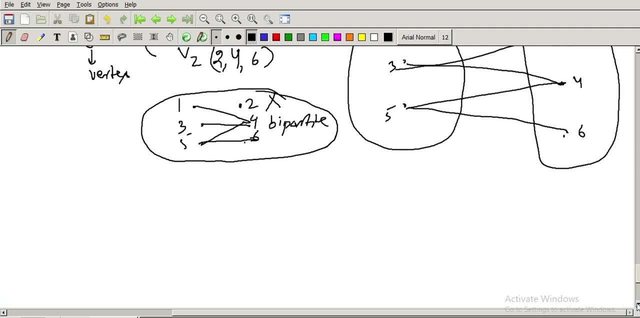 So we have a difference between these two bipartite graphs, right? So let's see, Okay, I think it's. I have some problem with that. Okay, now it's fine. Yeah, So let me write a definition for this complete bipartite graph. 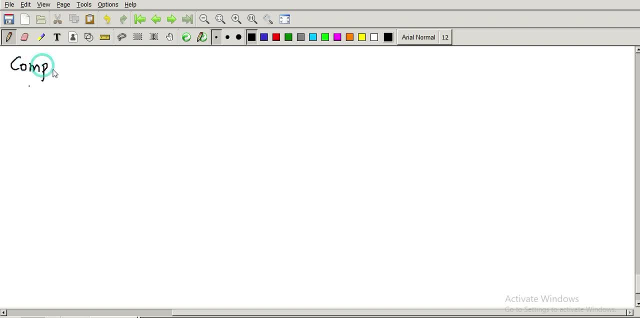 So complete bipartite graph. Okay, so, in complete, by bipartite graph, which is denoted as KM, comma M, right, And if you remember, the complete graph is Represented by KN, whereas complete bipartite graph is represented by KMN. 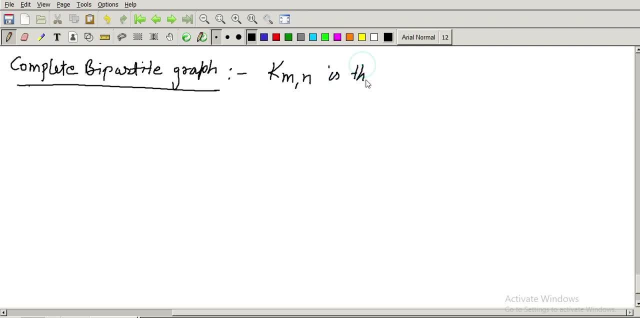 Okay, that is the graph, right, The graph that has that, has that, has its vertices, Partitioned into two sets, right, Like we have seen in bipartite graph, and two sets, V1 and V2.. Okay, V1 and V2 and such that. 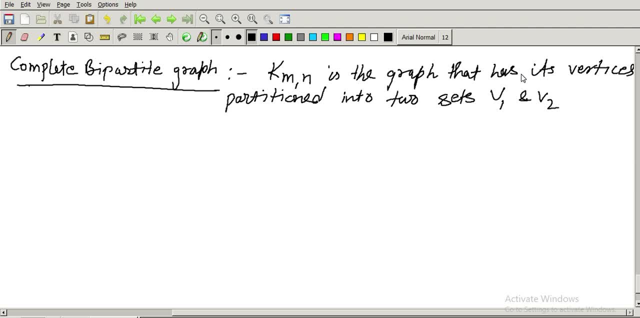 Such that, Okay, Such that there is an edge between two vertices right, Right. So such that there is an edge between two vertices Right. So let's understand it by example. So, first of all, what we have, we have taken 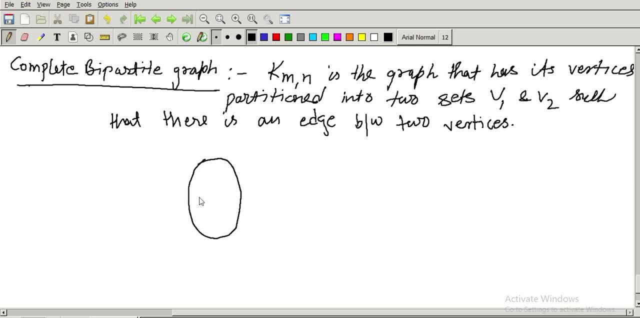 So Set Right, Like you don't need to draw this, like this is my way of representation, This, this, this. I write this one to three. This is one set, Okay, And V2 set. We have this set Right. 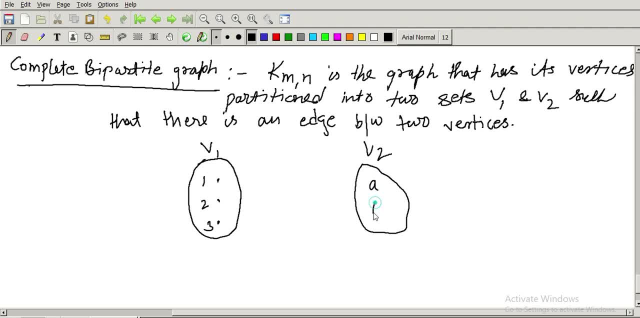 Okay, now a B and a B- okay, here we are. so okay, let's talk about these M or N numbers. so here V 1. M represents the number of vertices in set V 1, right, where n is the number of vertices in set V 2, right. so M. here the value of M is 3, here the 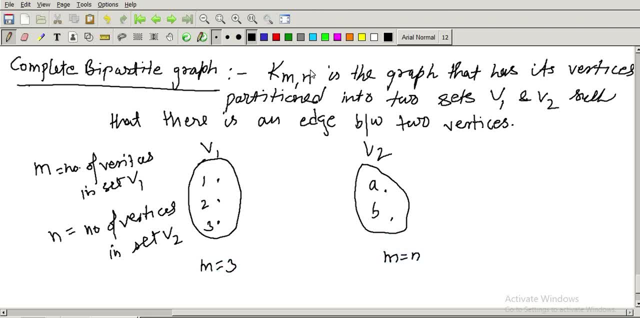 value of M is. so the definition says that we have some vertices which are 5, okay. 1, 2, 3 and a, B. there are 5 vertices. you can even number it: 4, 5, whatever it is okay- and these are partition into two sets, V 1 and V 2, like there, such that there is 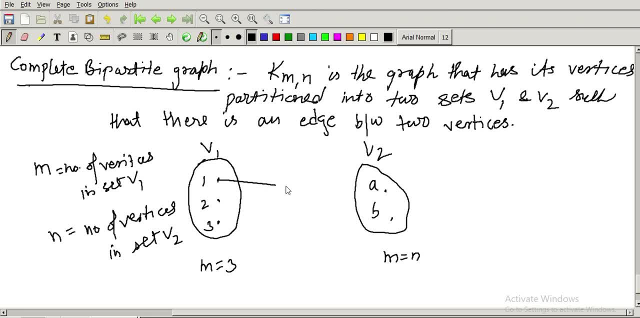 an S between two vertices. so A 1 is connected to A and A is connected to B, 2 is connected to A, 2 is connected to B, 3 is connected to A and 3 is connected to B. so this is your complete bipartite graph. okay, and complete means. 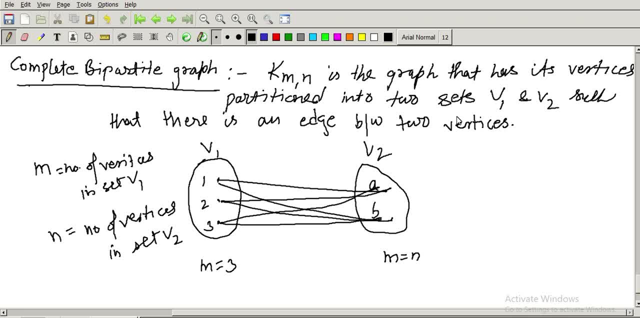 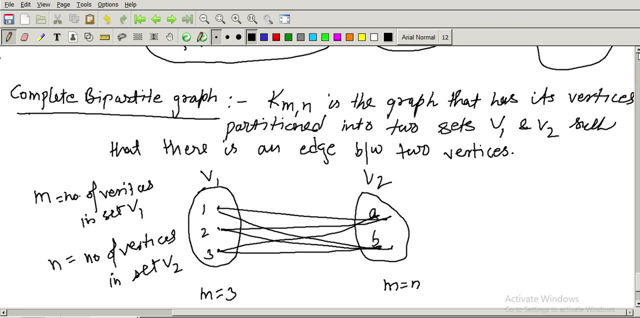 complete means. so this is your complete bipartite graph, okay, and complete means all the edges are all the vertices are connected to each other, right, sorry? sorry, vertex, vertex, who connected in exclusive right, but it was not the case when. when I write the definition for complete for the Bible telegraph, here we have this. 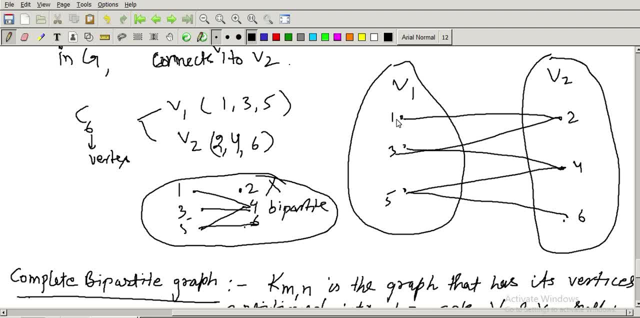 these two sets right, v1 and v2, so one is connected to but one is not connected to. for okay, so this, this, this is missing rate, this is missing. so if they present this, so this is the missing is right. likewise, 3 is not connected to 6, right 5. 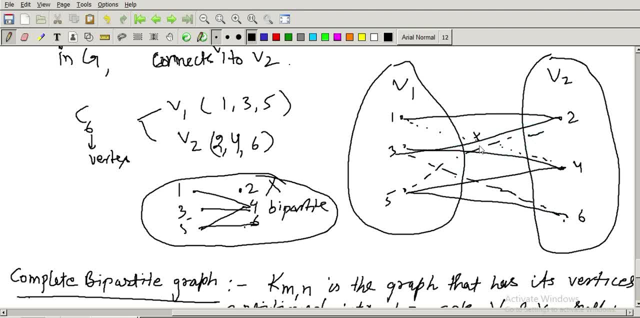 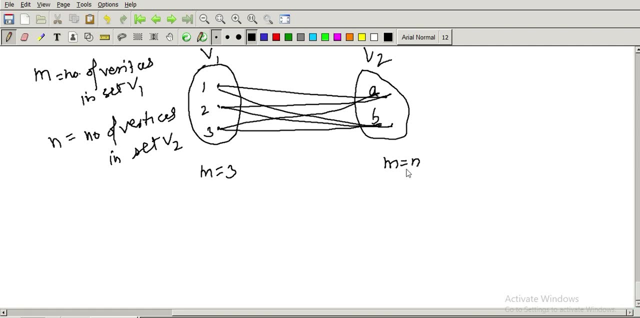 is not connected to be 2, so if I add these three edges in this graph, it will become complete bipartite graph. so there is a difference between bipartite and complete bipartite graph. right? so here we have written this. okay, so here is NH2. right, so we can see. 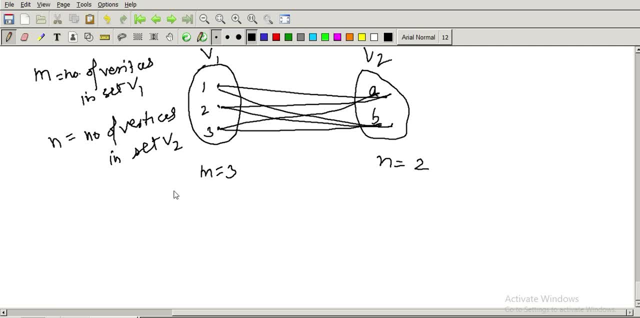 that if in there at times they asked you that in k 3 comma two, complete bipartite curve, that is a number of edges. so total number of edges will be your and cross n right. so three cross two will be six and put the number of 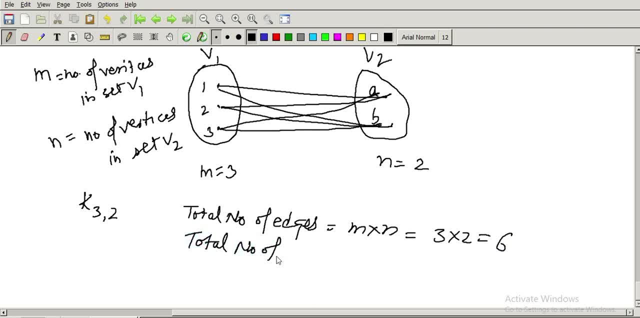 vertices. total number of vertices: c Hate VLT. number of vertices is your vertices: n plus n, which is 3, plus 2, which is 5. okay, right so. so let me add another page, right? new page, right, right, okay? so in exams they are not going to ask about the, the draw this graph or draw that. 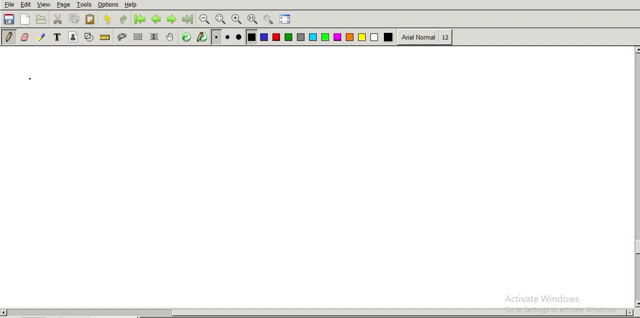 graph. no, what they are going to ask that we have in question. we have this complete bipartite graph in which we have 3 comma 4, complete bipartite graph. so they are going to ask: this is vertices, how many number are the vertices, how many number of pages, and draw this graph. they are not. 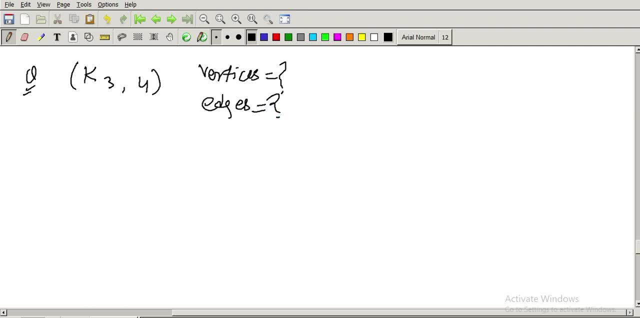 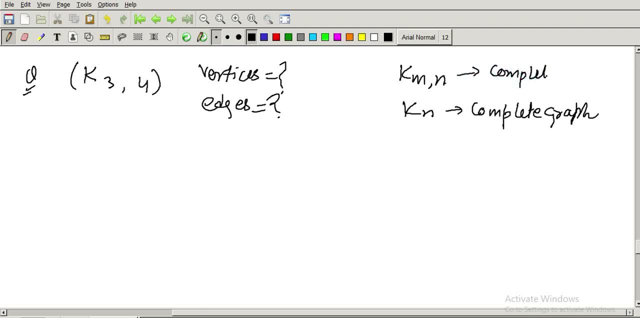 17 0, 17 0 17. complete by pertain. complete by pertain. okay, so let's move ahead quickly, because we don't have the, don't have it time because of your exam, right, okay, now another. we come to the graph. representation means how to represent. 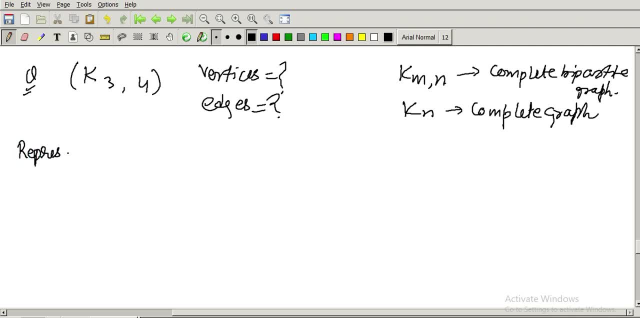 the graph, so represent graphs. so there are two ways to represent the graphs. okay, first is using your engines agents list, right? and second, the way is your agency matrices, right, agency matrices. so in exams that they will ask you questions about, to represent a matrix into these two forms, right? so how to represent this, right? so let me take an example. let's 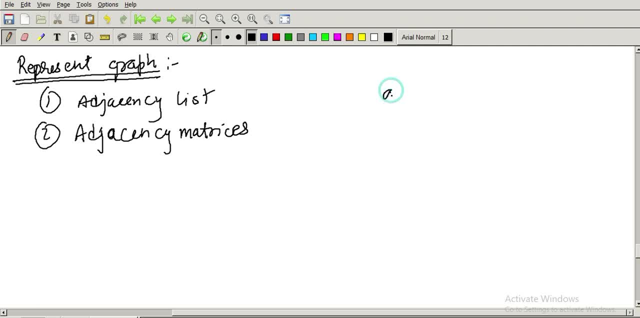 say that we have this graph right e, this graph, then we have C right p. here we have some right, we have this. we have this type of type of graph ID be this condition: C right a, and then we have A A, so C5 is weaker right, and so we we have gonosaurian. 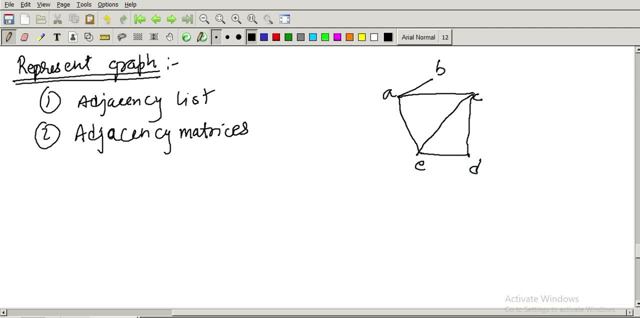 e. we have that concept that you03 have. it can be okay. so how to represent these graphs? right, using it, so, using an agency list. so so, let take this number as one, okay, so so what we have to do? you, we have to do a draw agency list, right? this is your list, in which we have two columns. we have 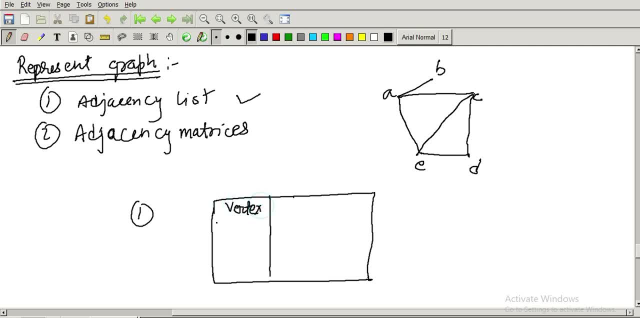 vertex here. then we have this adjacent vertex, right and sentimental vertex, right here the name of these words vertex. so we have a, B, C, C, D and E right, and then we have to write here the adjacent vertex to these vertices. so what is, what are the adjacent vertex to a? so to a, we have this bead. adjacent to a, C is, ad is. 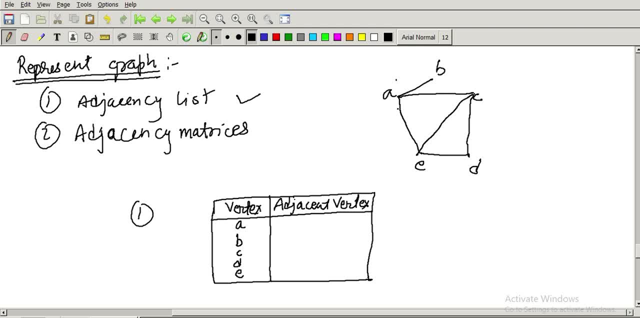 to a and E is also adjacent. so for a we have three adjacent vertex. so what are this there? b, c, c. this is your list representation of a graph. If you are asked to represent a graph in a list, then we will do this. Let's take for B. For B, we have one adjacent, which is 1.. For C we have A, E and D, So we will write A, E and D. 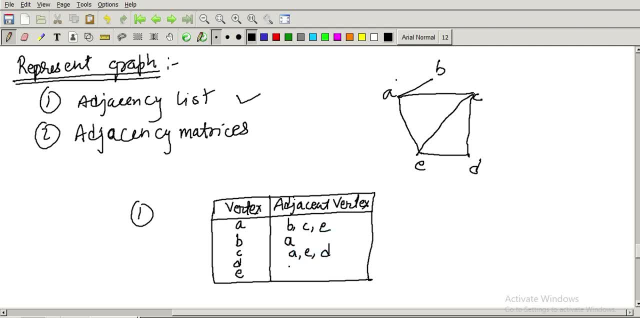 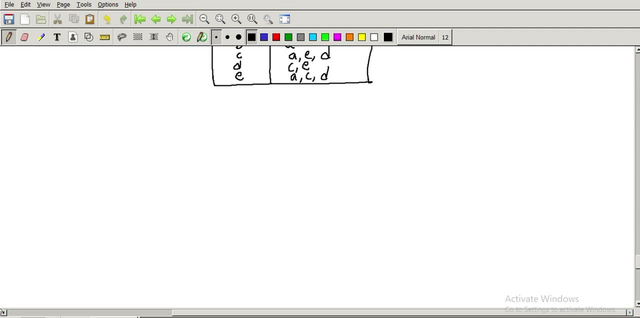 For D we have C and E. So for D, we have C and E, For E we have A, C and D. So this is your list representation of a graph. So let's take another example. Let's take this graph A. 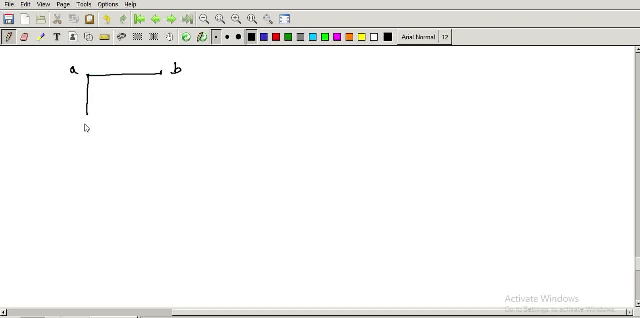 B, C And we have this D Alright. So, using adjacent vertex right adjacent vertex, what we have to do? we have to Sorry, sorry, sorry, Adjacent, not adjacent vertex. The second representation: The second representation is your agency matrix right. 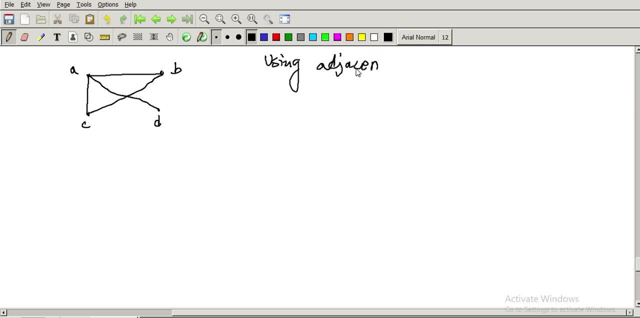 Agency matrix right. So in that we have to make a matrix in which we have this type of representation, We have this A right: A, B, C, D. We have this: A, B, C D. The formula is: let's say: in a matrix, you know, let's say: if a matrix, if we represent matrix as A. 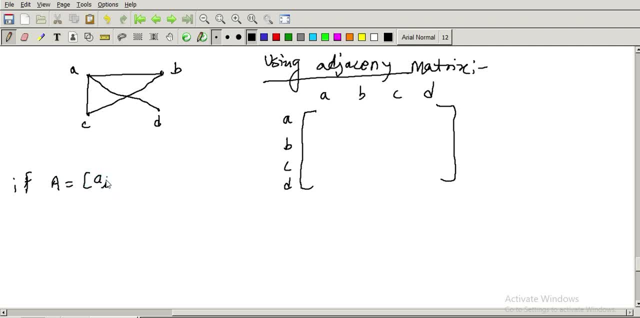 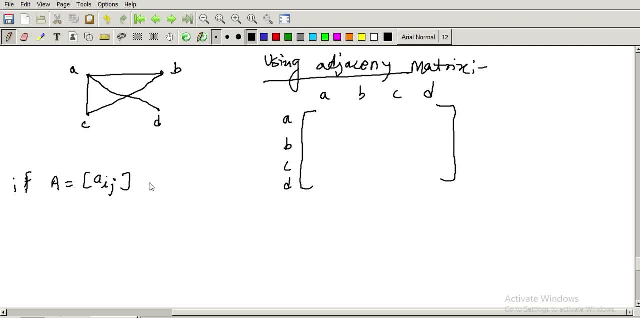 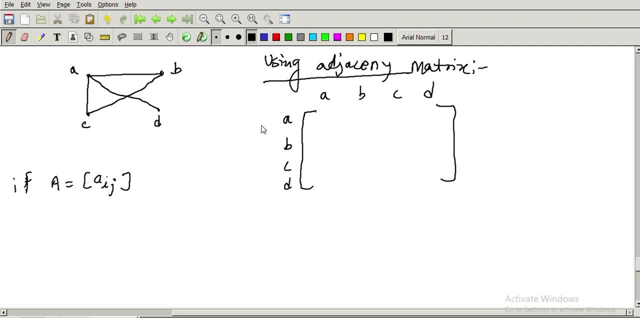 A, B C D, A B C D, Right, So what we have to do is that We have to write in this representation the matrices. So we have to do it in the first case. So now we are going to sum up the vertices of the matrices. 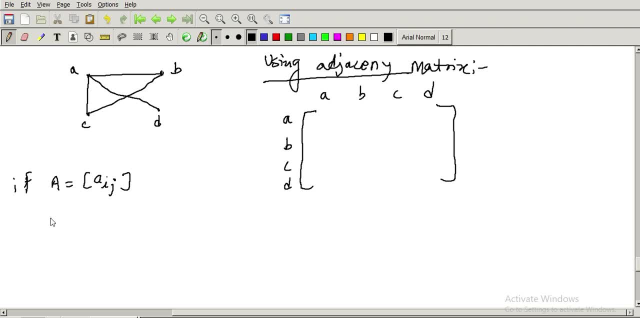 So number of rows equals 4 columns. if, if I say, is an s of G in this graph, so we will write one, right, okay, so we will write one. so we will like one man. there is an edge between ing and zero, otherwise simple. so, for example, between a to a, there is a s between a to a, no, so 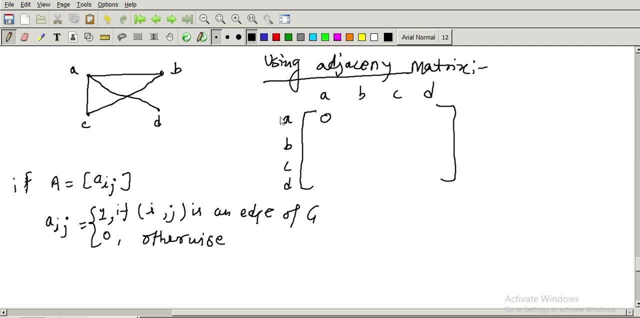 it will be zero. there is an edge between a to b, a to b. yes, we have an edge between a to b, between a and b, so we like one because of this definition. and there is an edge between a to C. yes, we have. this is two. we have an edge between a and d. yes, we have, so we will let one here and for. 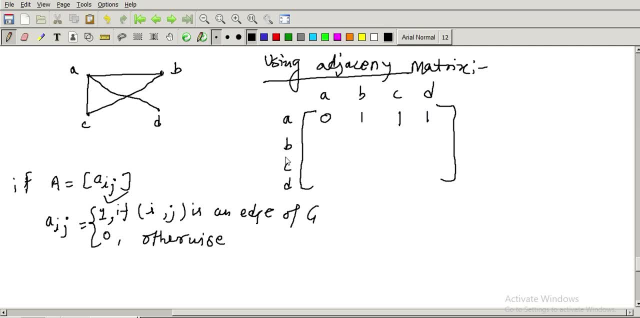 B. likewise will be for B. so for B to a, we have an S for B to B. we don't have for B to C. we have an S for B to D. we don't have because B to D is missing. then say for C, let's take for C. there is an edge between C to a and B, so we will write. 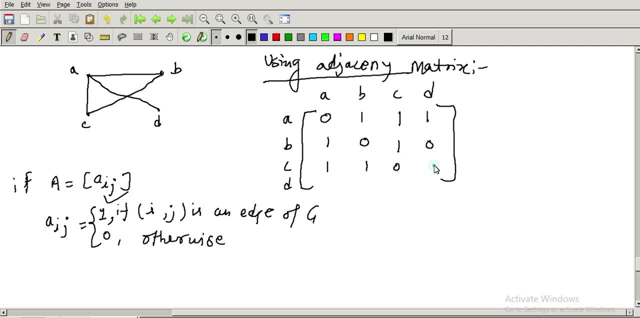 one edge between a to d. okay, one one here, otherwise it goes to d. we have only one is between a to D, so we will write one here, right? otherwise you will. so this is your representation of right graph using agency matrix, right? so what if we have this? 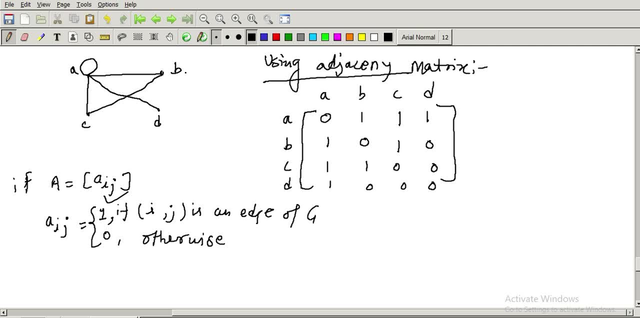 okay, I change to this: if we have some loop, right. so what will be right here? we have to make some changes because there is an edge between a to B, so we'll take one here, right? so it will be the case when we have this direction, right? we? 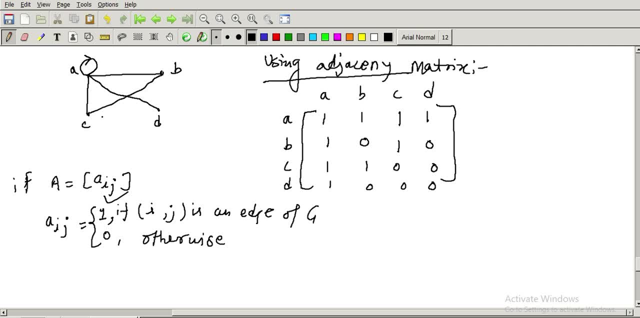 have this directed graph because it was the undirected graph, so we can represent the directed graph as well. so let's take an example for that. we have this, we have this, we have this right and we have this. okay, so this is the undirected graph. so 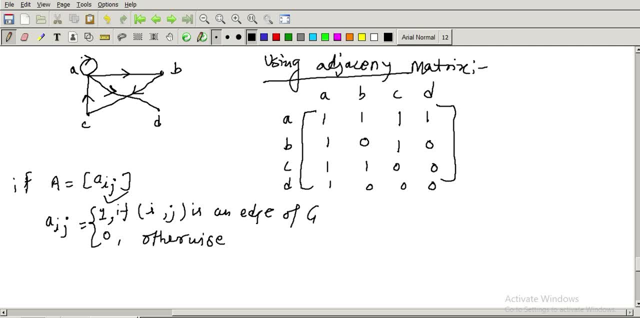 that matrix will be changed now, because a to a, yes, it is going from way to, and terminus at a, only so it way. s1, a, twenties: yes, a to c, 80c is not because it is c to it. so a to C will be in gt right. and then we have a to D: yes, we. 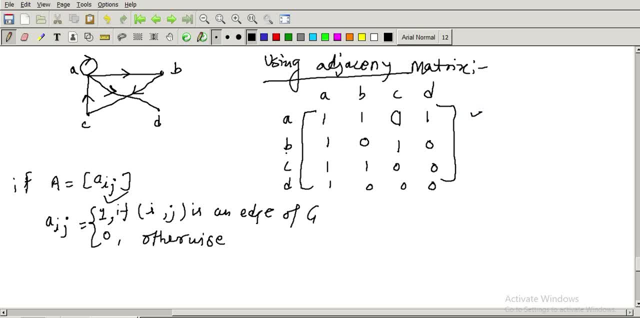 have a duty, so it is correct for this a, then this represent for b, so B we have only B to C is because this is a I'm good euro. also, somebody says from – AM the так for the micro plane. let's like, let's say, I'm person for this ego. this is in format okay, except inonsense. so this actions are: 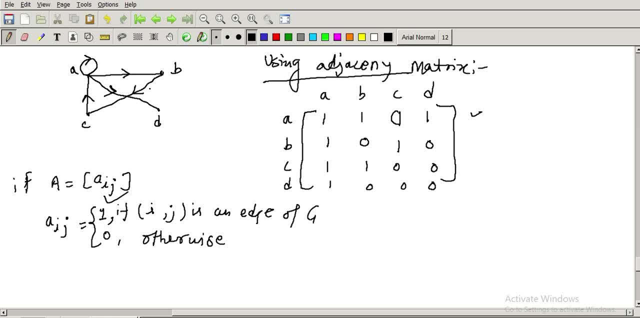 this is dark, it to you know from B it is, it is going okay and it is inviting to our speed. so the outgoing, as is from B: right, this is only C, so that we have only one here, otherwise all the for all the vertices will like geo. for C we have. 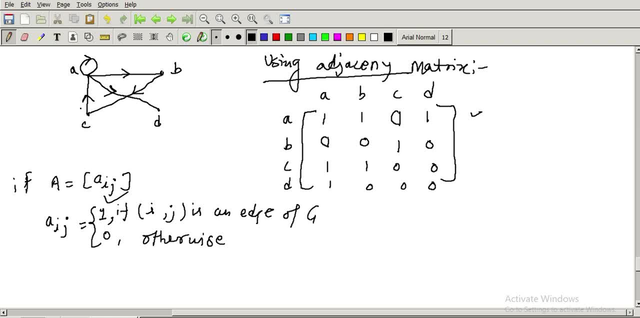 only one outward. okay, so we have C to A, so we will write C to A one, otherwise otherwise you so. so so let me get me deleted right from here one, otherwise zero right. C to C to A. okay, C to A is one, otherwise we let. okay then for D, for. 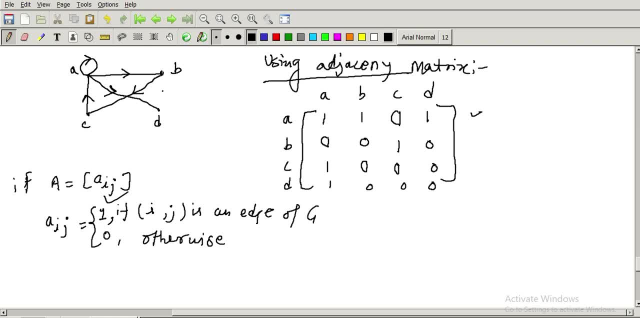 D. we don't have any as outgoing from from. okay, so we will add 0 0 0 0. so this is the way you can represent right using the agency matrix and director of Antarctica graph and if, if there is an doubt, you can ask me. okay, now. okay, let's talk about another important topic, which 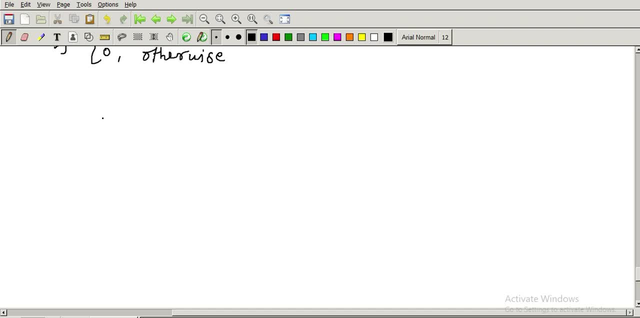 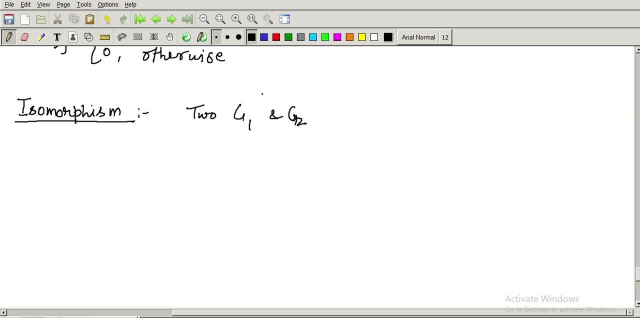 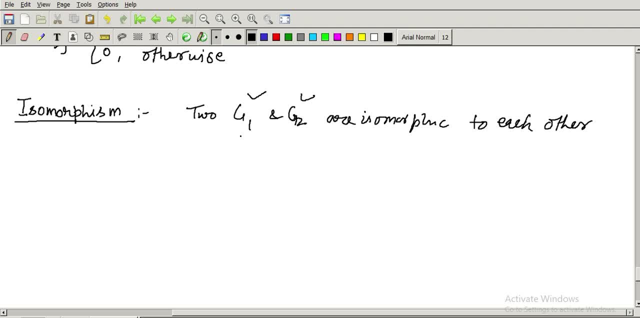 if they are one two. one and one two function. okay, one, one and one two function. so, uh, it will be complicated to understand the one, one and one two. uh, sometimes in the, in the two graphs, if they're given. so what we have to find, i'm just giving a trick or or simple solution for this. 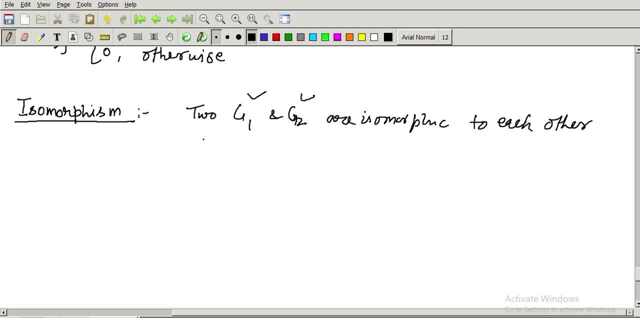 which is to each other, when we have these three, three conditions: first, the number of ages. okay, number of ages are same. number of ages are same, obviously, in in both the graphs, in both the graphs, both g1 and g2 right. second, a number of vertex. okay, your number of vertices? 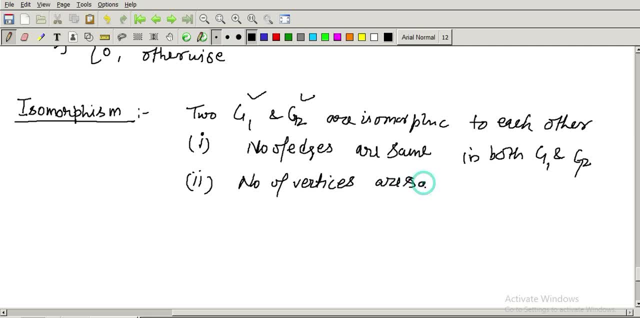 are same, right are equal or same, whatever you say, in both g1 and g2. right and number of degree: okay, the degree, okay, degree of vertices are same, okay in both g1 and g2. and the next uh, which is, are that adjacent vertices must have the same degree, right? 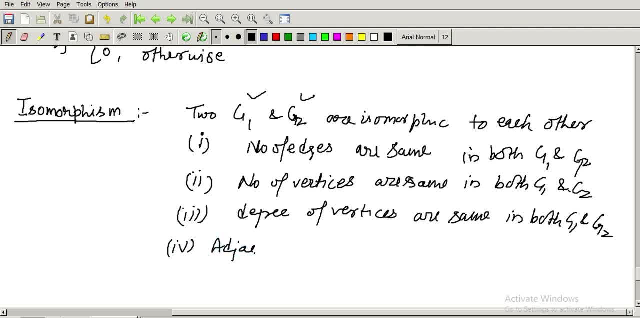 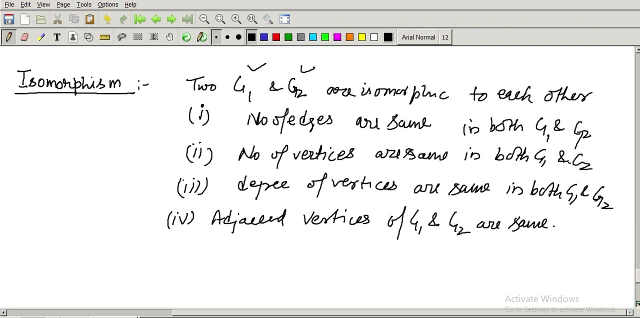 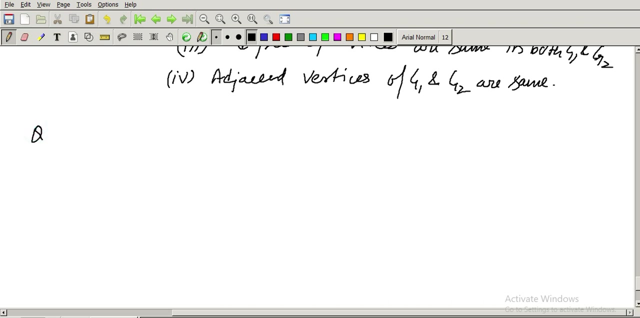 fourth is: adjacent vertices are same. adjacent vertices, right adjacent with this. vertices of g1 and g2 are same. okay, or whatever臥, it must be same in in both the graphs, right? so let's take an example for that. so we have this uh graphs. they have asked in your, in your exam, that. 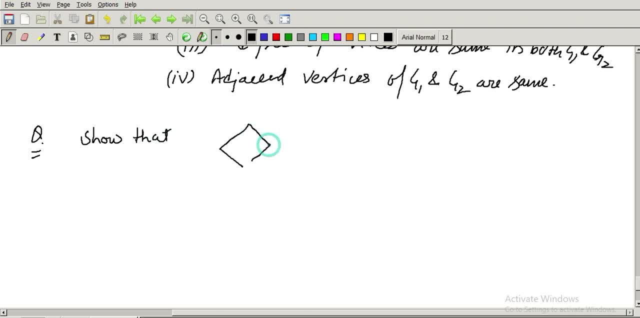 so, and these two graphs are- are isomorphic to each other. these two graphs that i am just writing here- a, b, okay, okay, a, b and c, e, and one, two, three, four, right. so if this is the case, it it okay. okay, one second. if i take another example, right, i take another example because 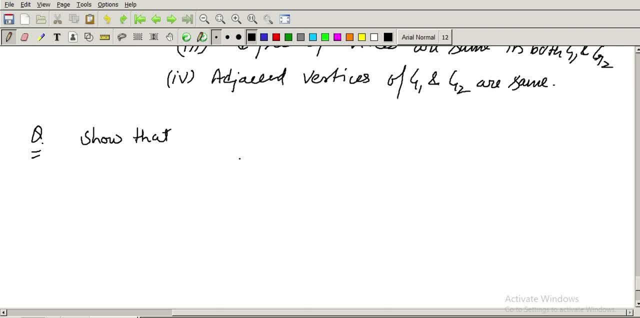 let's take another simple, very simple example. the example is like this one: this is the example. right, we have this: uh, u1, u1, u2, u3, u4. right, we have here another graph which is like this: so we have v1, v2, v3, v4, and this is your g1 and this is your g2, and this, this is that. 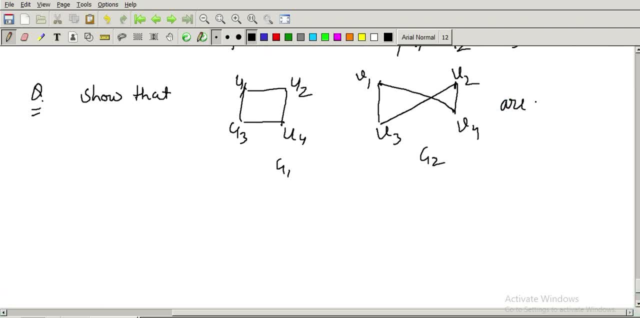 identify that, if they are there, they are isomorphic to each other and not, okay, isomorphic to each other. i'm so morphic driven, isomorphic to each other. so for, to prove that, what we have to do, firstly, the number of ages, number of vertices, number of ages, number of ages, number of 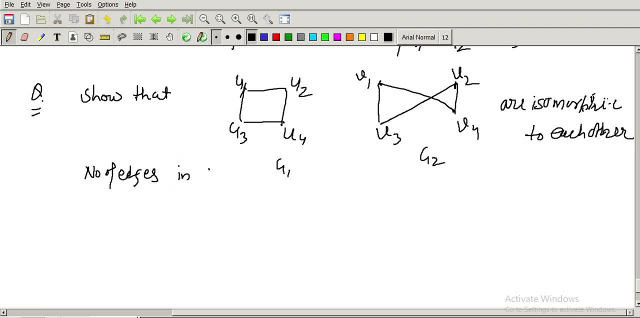 ages in g1 is 4, right, 1, 2, 1, 2, 3, 4, 4 edges and number of ages in, let's say in, in in g2: 1, 2, 3 and 4, 4 edges. number of vertices: vertices in g1, which is what. 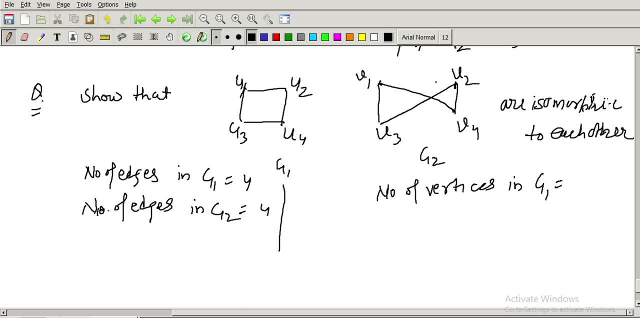 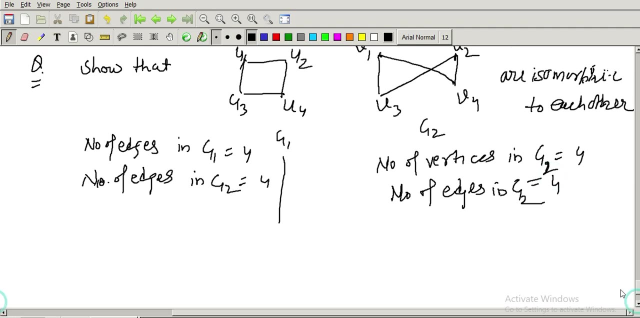 this is a 4, 1 V, 1 V, 2 V, 3 V, 4. number of ages is also, which is 4 right, and then calculate the degree. so the degree of u1 in this graph is 2, number of degrees in u2 is 2, the degree of vertex u3 is 2, and if you 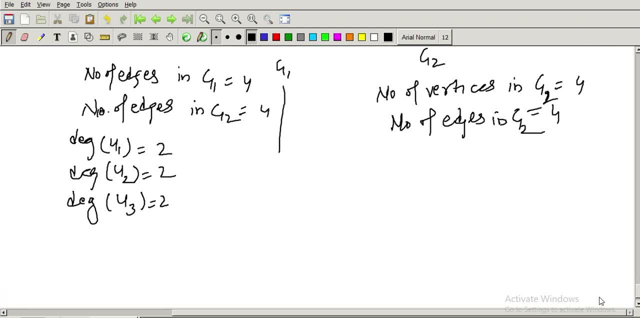 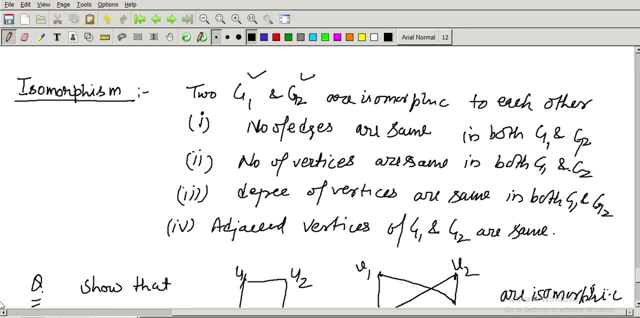 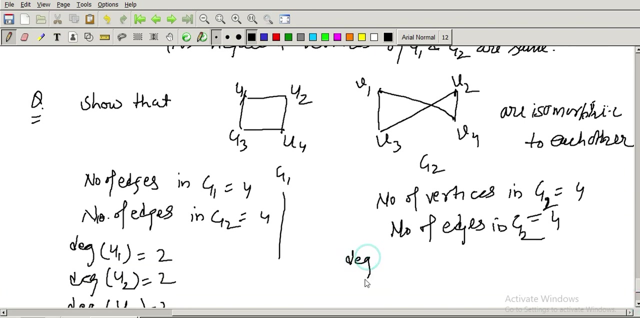 don't know about the degree and then find out my first lecture right. so degree of u4 is your 2. so all the vertices are the same degree in g1, right 2, 2, 2 and for v1, for this to say about this graph, g2, the degree of v1 is 2. degree of v2 is 2. 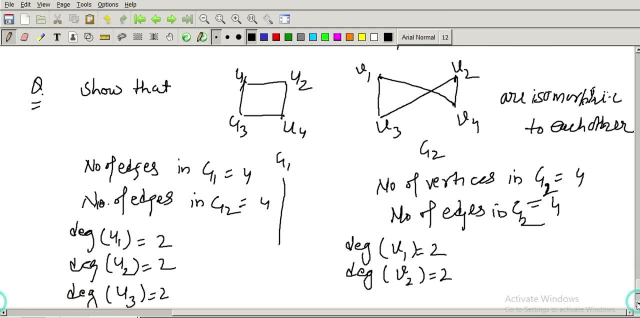 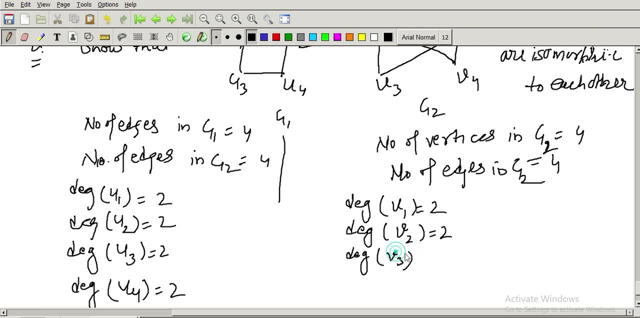 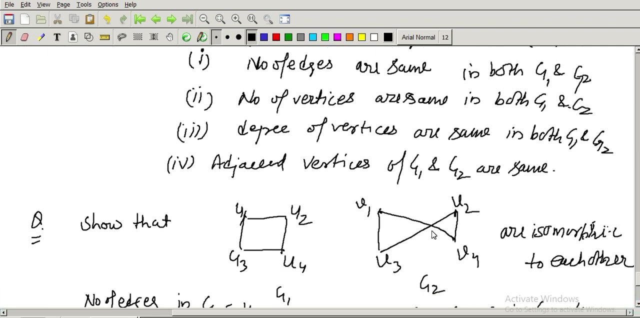 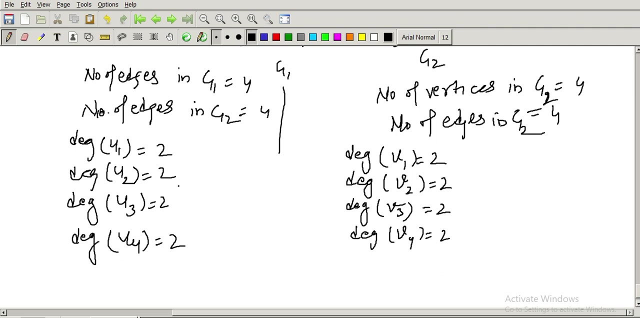 right degree of v3 is saya. if the last is the adjacent vertices out the same day right. so here we can see that doesn't decrease it. I say this existent degree very. these are basically. so we can see that we can see that these two to two graphs are isomorphic because 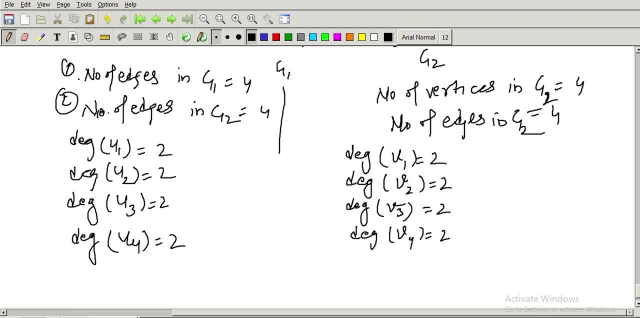 this is your first condition: number of edges. number of edges or the number of edges, number of vertex right. so here I have written: number of vertices right. number of vertices: g1 is 4, edges is 4 and g2. we have vertices 4, edges 4 and the. 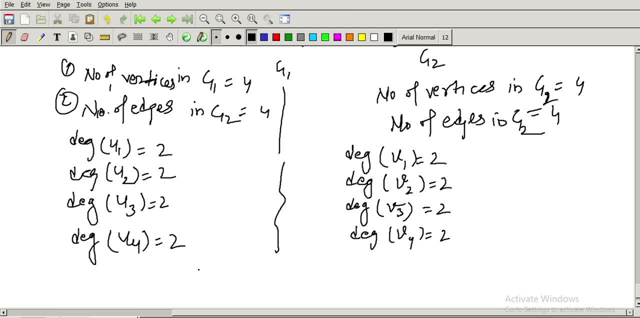 degree are the same. okay, so we can say that the g1 and g2 isomorphic. we see many examples when the two groups are not isomorphic. so let me take another example: when we have to prove that these two graphs are isomorphic or not, right so? so this is your example, right, in which we 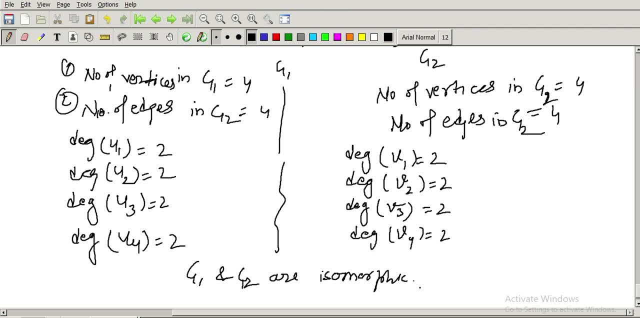 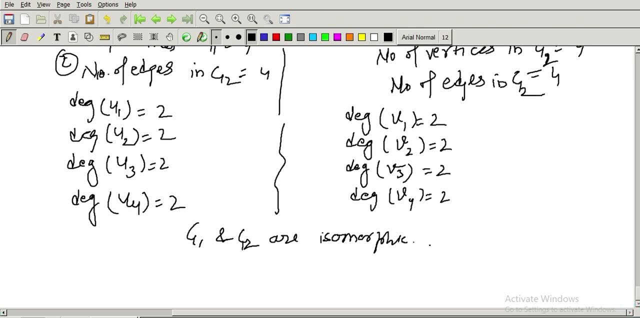 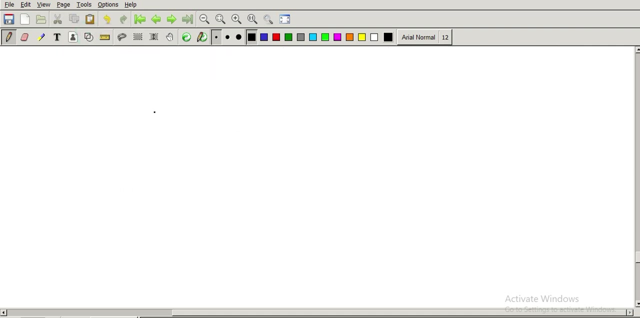 can say that these two graphs are not isomorphic to each other, and there are various examples, basically, but I take this example to you, which is like this, so let me add another piece here. okay, now we have this. this graph- actually the graph is your, this is your graph. 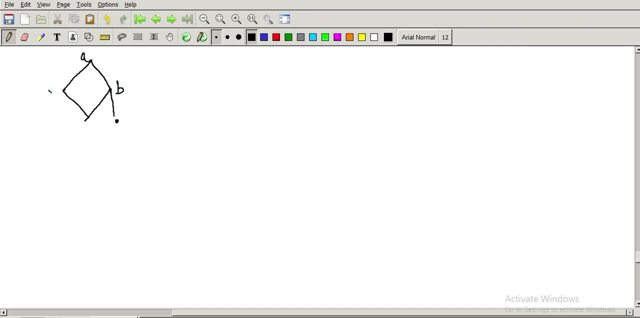 so we have this: A, B, E, C, D, like that, okay, and then we have: this is your a's or not, this is your else, and we have these edges. then we have this, another graph, which is this: great. so here: 1, 2, 3, 4, 5, right. 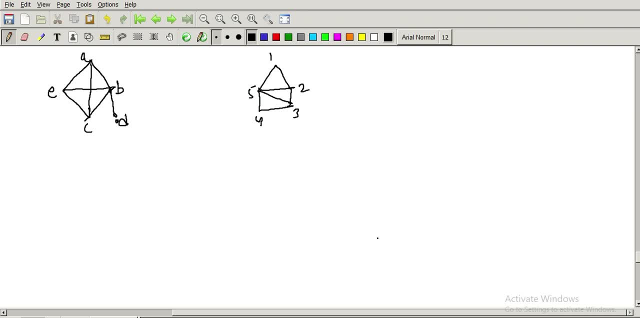 so these are two graphs, right? okay, now let find. the number of vertices in this graph is 5. number of vertices in this graph is 5. number of ages in this graph in this is graph One, two, three, four, okay, five, six, right, it is in this: one, two, three, four, five, six, okay. 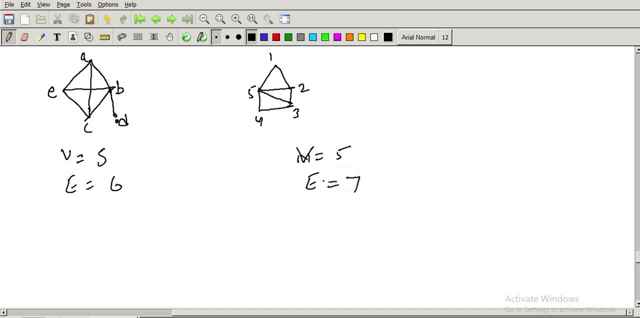 Yes, it's sorry, ages are seven actually, Because here you can see one, One, two, three, Four, five, six and seven, right, so number of edges are seven. So we have this, seven edges here, seven edges here and the degree. let me count. the degree for a is, degree is. 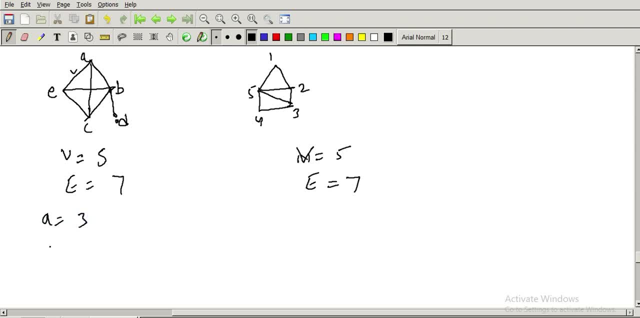 Three, one, two, three For B, We have degree four. For C, We have degree right. three for D, We have degree one. For E, We have degree three and for this graph, full degree One, we have two. degree of one is two, degree of two is your.